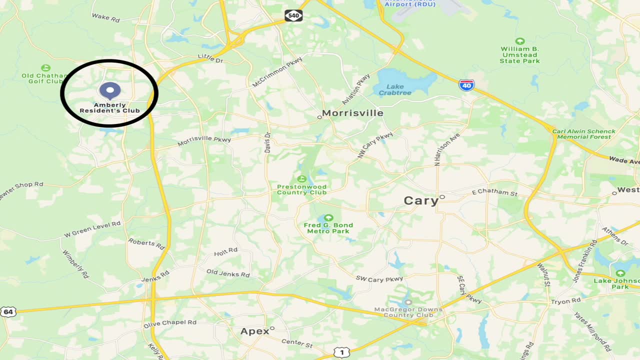 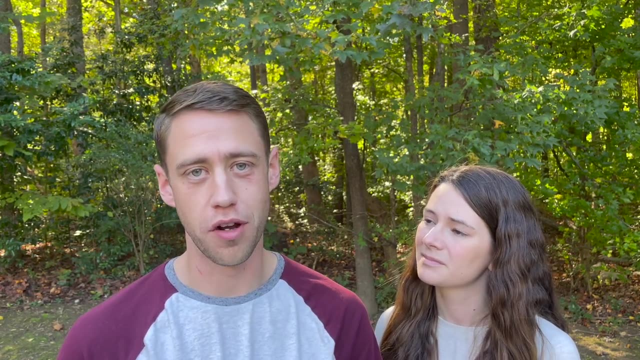 significantly closer to the Durham side of Cary. So, being close to the Durham side when it comes to amenities, you're not far from the Durham side of Cary. So if you're looking at a map, you're not far from, obviously, downtown Durham. if you enjoy to go downtown Durham, You're not far from a place. 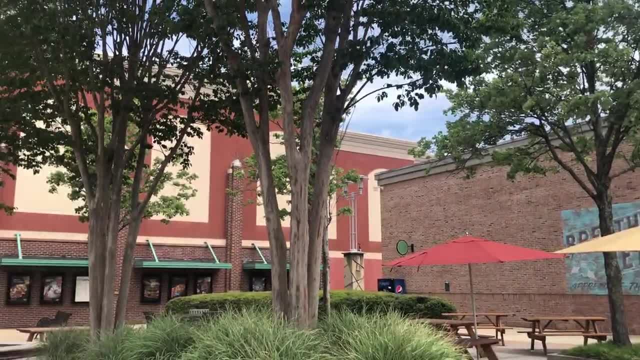 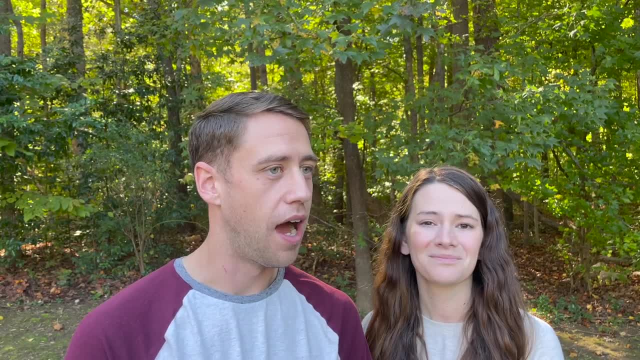 called South Point, which is a large shopping center on the south side of Durham. It's a mall. it's got restaurants and like outdoor shopping. It's a beautiful mall. Yeah, it's really nice. You're not far from Jordan Lake. If you like outdoor activities, Jordan Lake is a really 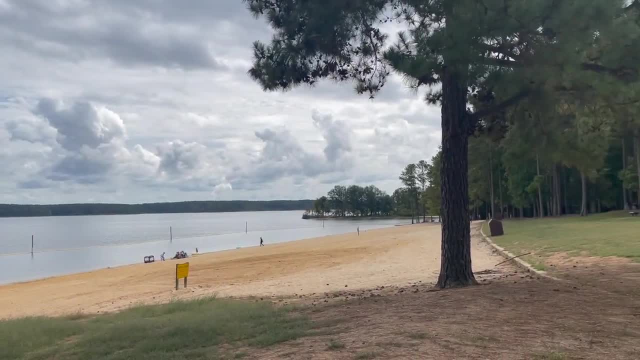 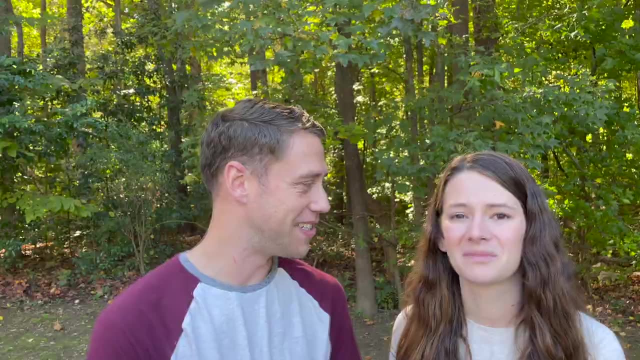 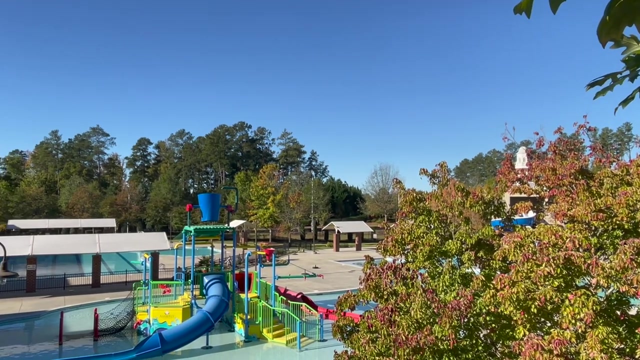 really really cool spot. Yeah, so Amberley, as far as neighborhood highlights, just a really fun neighborhood. So if you look at their community center where their pool is, it's just the water slides on there are really neat. Like I wanted to jump on those water slides, They were really cool. Yeah, it was. 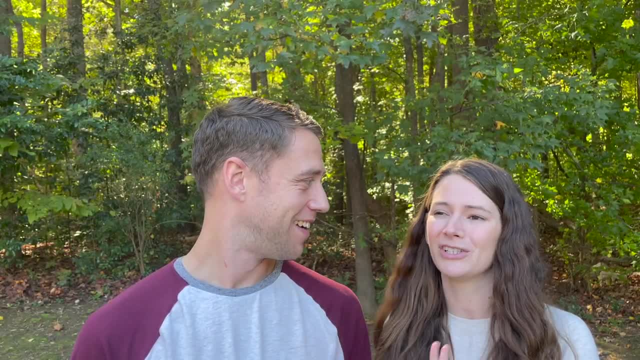 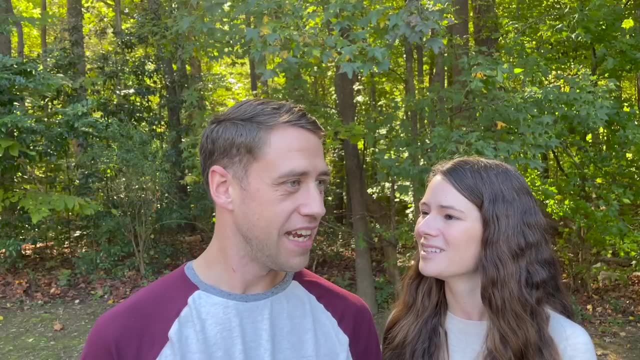 like a water park or something You know. they had like the just a traditional, you know big slide, that they had an area like a climbing structure- Yeah, so it was really cute. It was so cool. Yeah, so they had that There were some walking trails. Just, I mean the neighborhood in general. 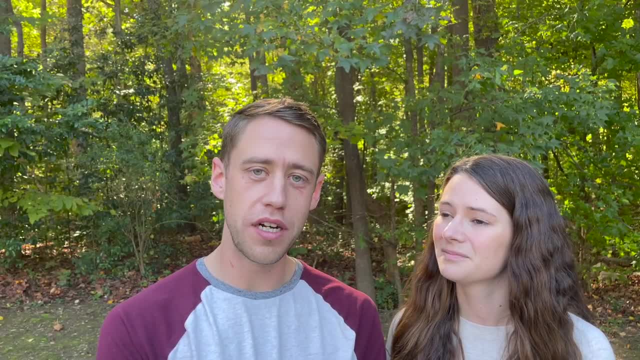 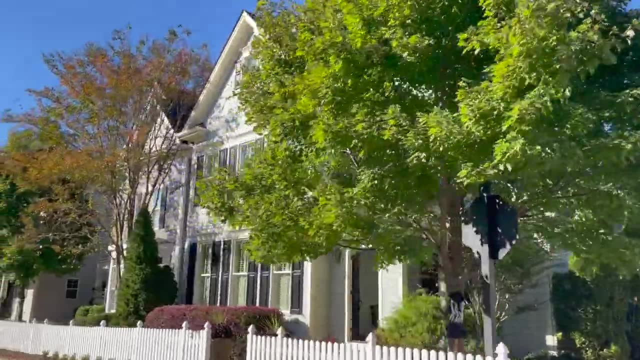 when it comes to the housing, houses were really close To one another, but it didn't feel, which typically I don't like. I don't like when houses are, you know, stacked up on top of each other. But I don't know, they pulled it off. They pulled it off Well. 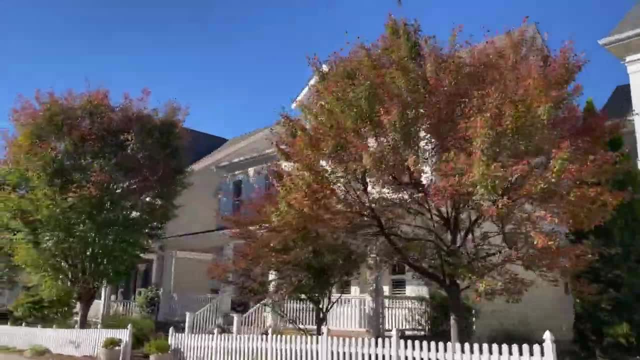 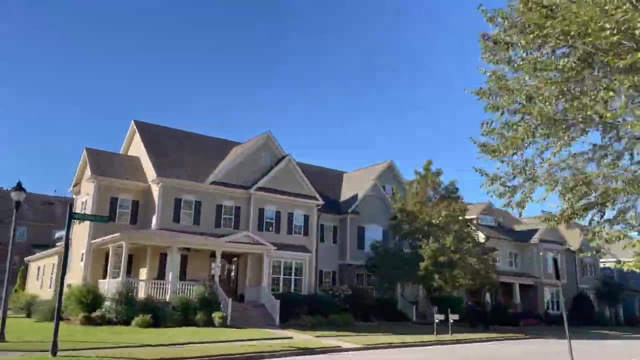 it looks nice the way that they've done And there are differing lot sizes So some of them are like kind of like rose style houses, So the garage is like in the back and those are a lot closer together. But then there was houses that weren't in that style, that have a bigger yard, So kind of. 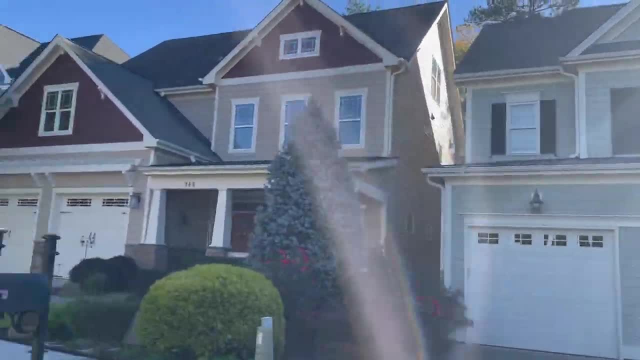 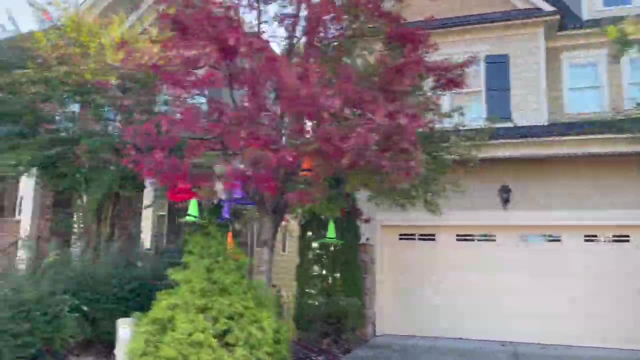 depends on which home you chose to be in there. So I have to say, if you just drive through the front part you might think, oh, these lots are way too small. But if you go into some of the further back sections you realize there are opportunities for. 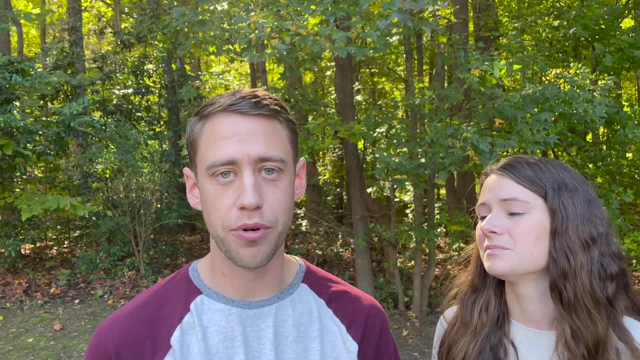 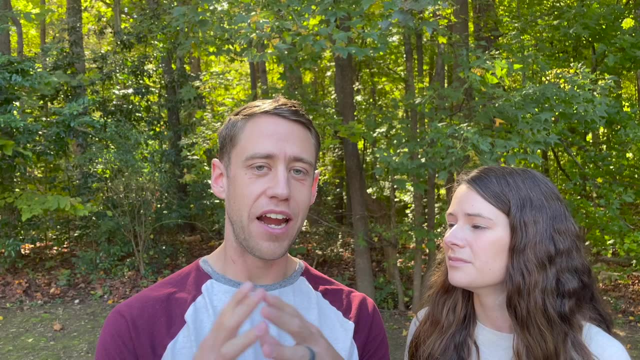 bigger lots, Yeah, yeah, And as far as price points go, in Amberley you're looking on average in the mid or in the low fives, excuse me. So if you're looking at Cary as a whole, just for the rest of 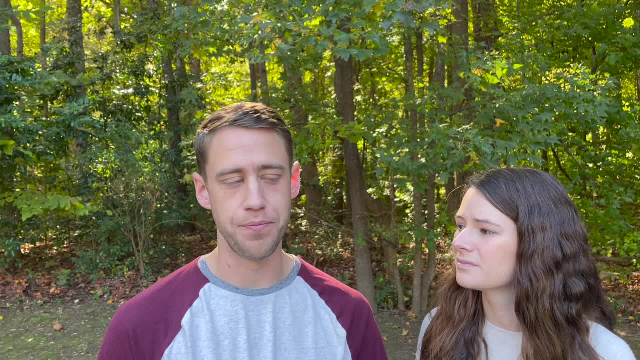 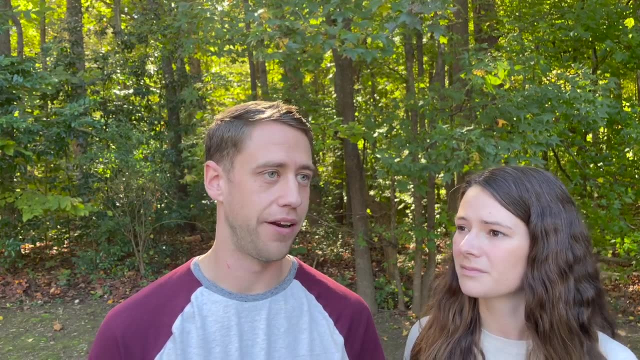 the video, Cary as a whole is in the mid fives And so to be low fives puts it pretty much at the average price point that you're going to find, And Cary, but for I mean for that price point, I mean you're, you're, you're getting, you're getting. 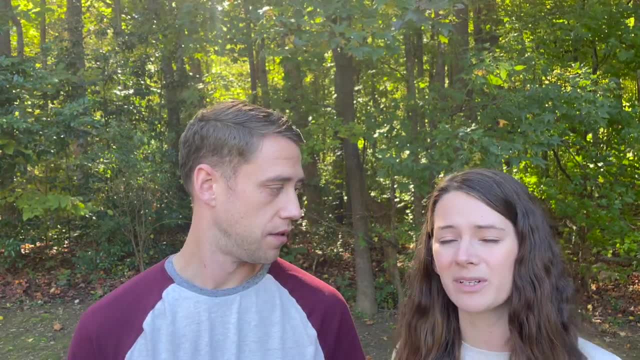 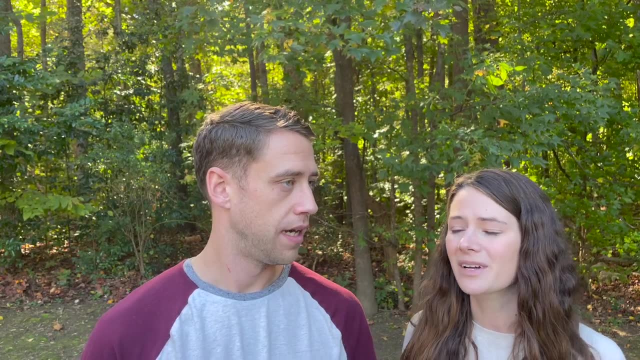 a loaded neighborhood. Yeah for sure, And it's such a big neighborhood. So there's like town homes that are cheaper, on the cheaper side of that, like in the 300s, And then they have homes that go up to like a million dollars in Amberley. So obviously that's a pretty- uh, an average. So 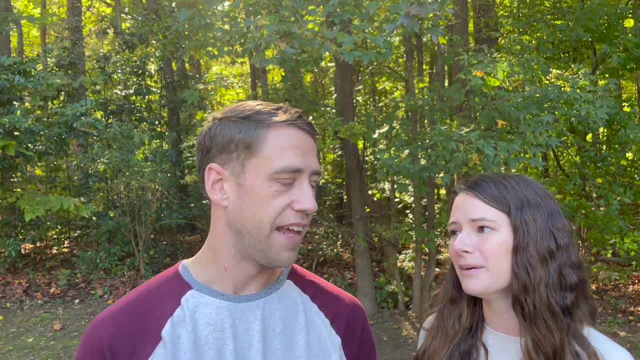 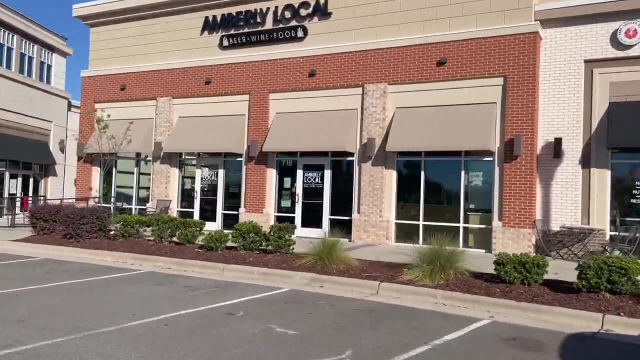 you might see stuff significantly less or more, depending on what home you're looking at. And there's a shop, there's shopping, there's like a shopping center pretty much in like the center square, I guess. It's right near like where the pool and stuff is, And there was restaurants in. 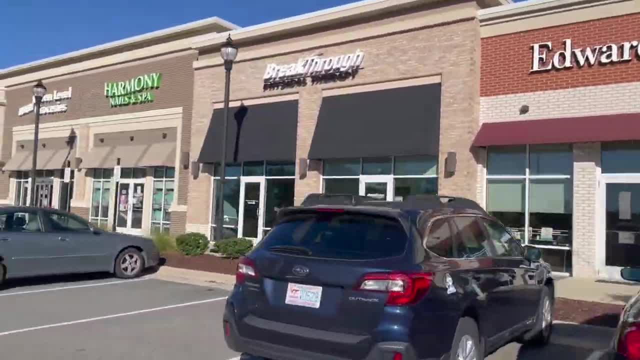 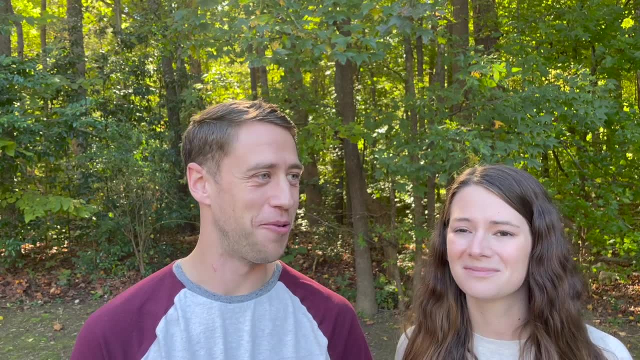 there. There's a retirement community in there with a really nice retirement center. Yeah, And that was called Carolina Preserve at Amberley. Yeah, Yeah, Folks were driving in their golf cars to the retirement center. It was cool, It was really neat. It was really neat The. 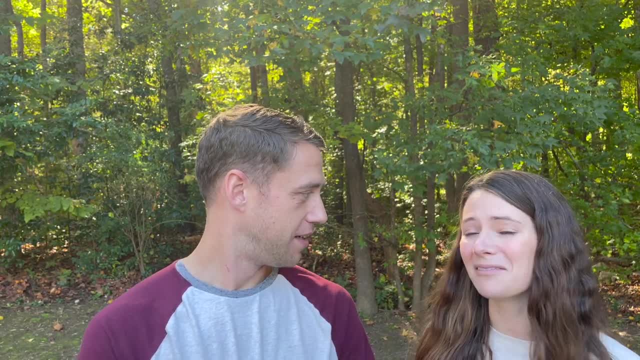 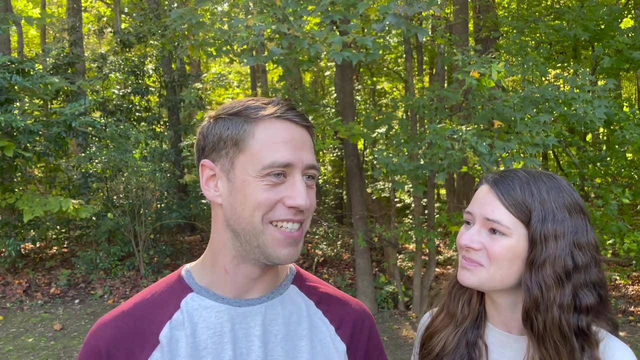 retirement area had like an indoor pool and I'm taking it. They must have like a lot of stuff going on inside the community center because there was a ton of people out there. I think they had some. is it bocce ball? Yeah, Yeah, They had some bocce ball lanes on the backside It was. 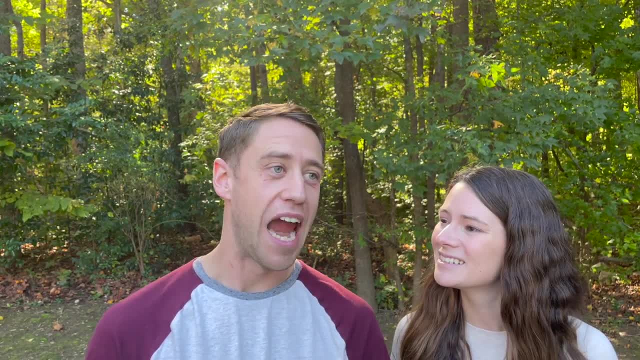 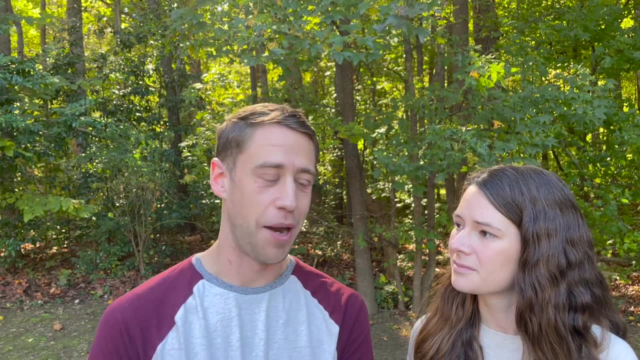 really cool. It was a cool spot, Yeah, Yeah, But as a whole, Amberley, Amberley- honestly, all the neighborhoods we looked at and out of all the neighborhoods we're going to talk about today, Amberley was my favorite. Yeah, I think it was in my top two. It's hard for me to pick one. 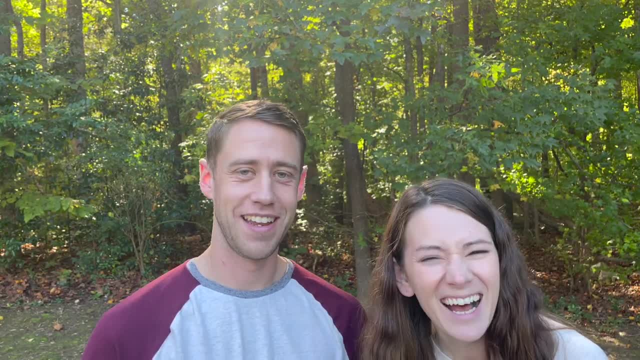 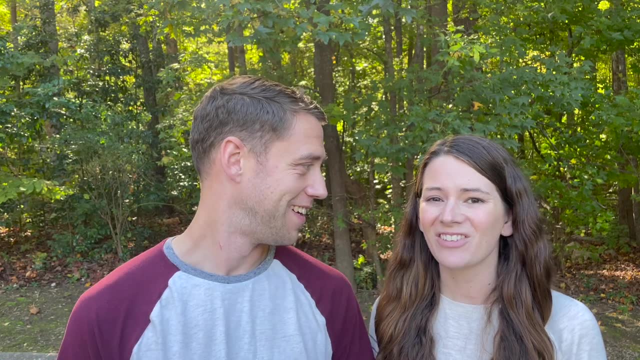 but it is a really good one. It's great for family. I like different ones for different reasons, but if you have like young kids, I think Amberley is awesome. Yeah, So the second neighborhood on our list today is called McGregor Downs. McGregor Downs has a completely different 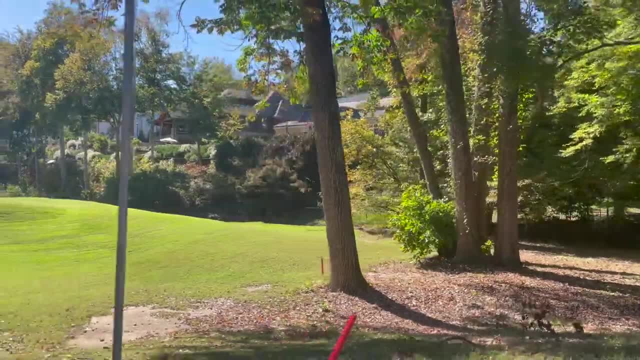 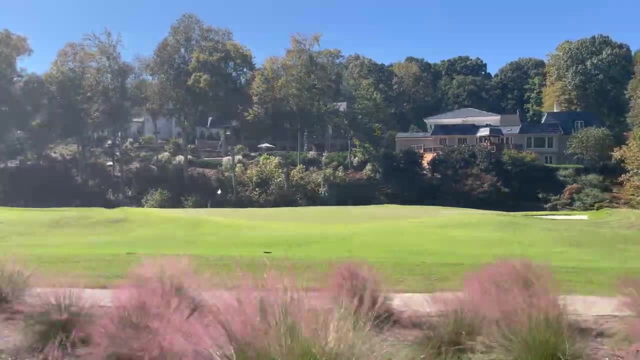 neighborhood. This to me feels very like. it's a country club type neighborhood. Yeah, There's a golf course and, um, you know, the homes are more stately, Um, I would say, but it was absolutely beautiful driving around for sure. And as far as location goes, uh, McGregor Downs is going to be. 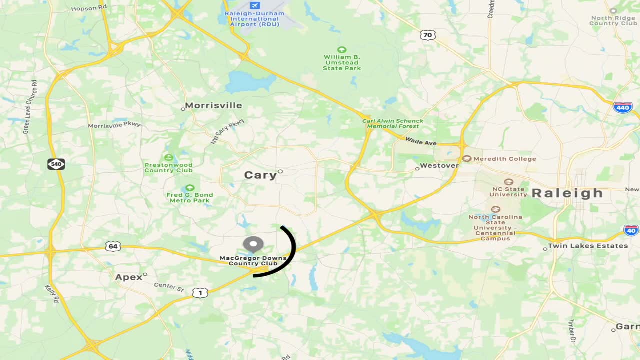 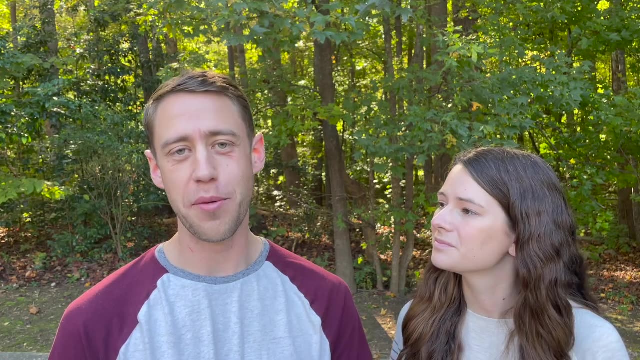 on the South side of Cary. Um, it's near. there's a couple of shopping centers nearby. Um, it's near a place called Coco booth as well, which is outdoor amphitheater. Uh, some of the other neighborhoods we're going to talk about is also near that as well. So, uh, just some amenities. 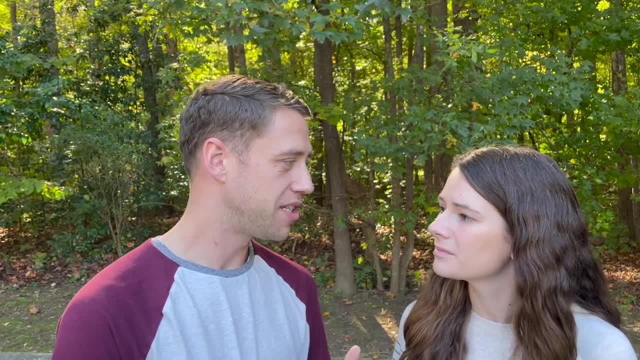 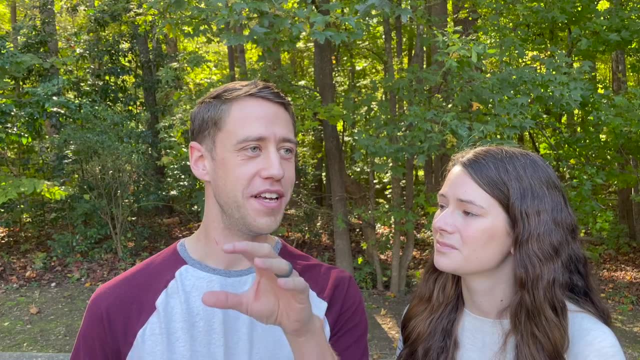 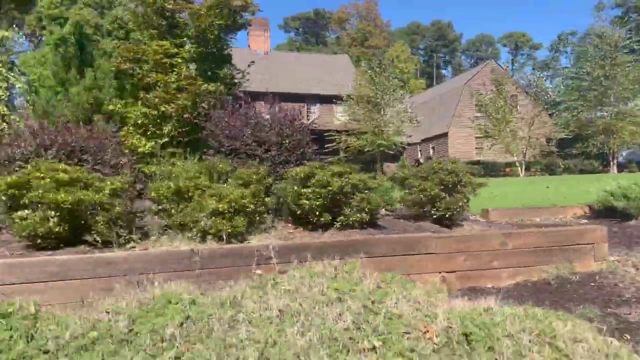 they're close by uh McGregor. but yeah, when it comes to like the housing style, McGregor was unique because every house was totally different, Like there were homes in there that looked like a log cabin and then there were homes that were like super modern. Yeah, Very. 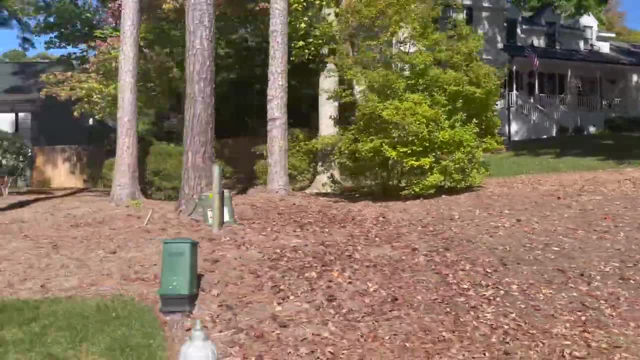 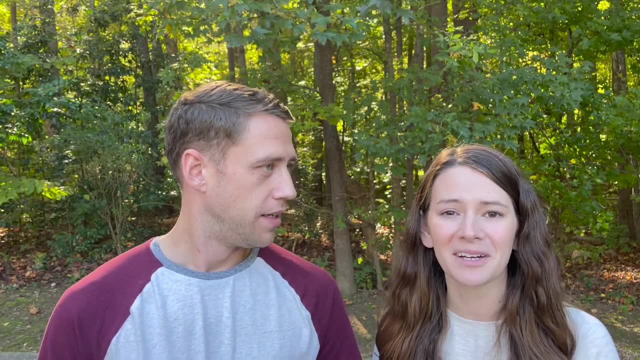 modern And then I, yeah, it was just, it was so, it was so different and unique and I don't know that was really cool. Yeah, I like that, It's refreshing. Um, there's nothing cookie cutter ever about McGregor Downs, So if that's something that you just want your house to feel unique, um, 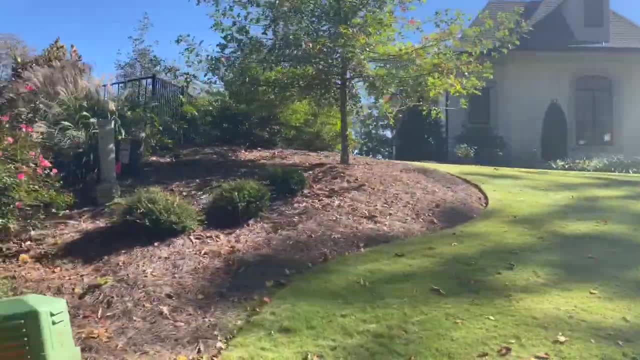 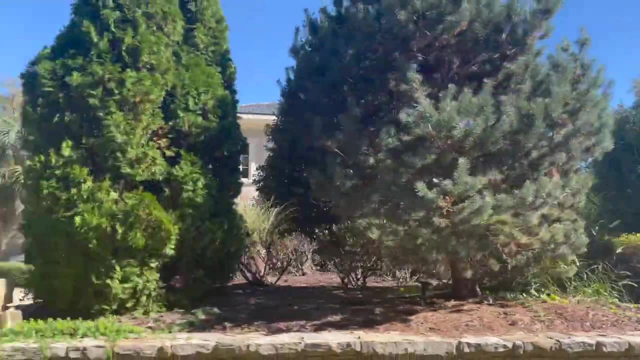 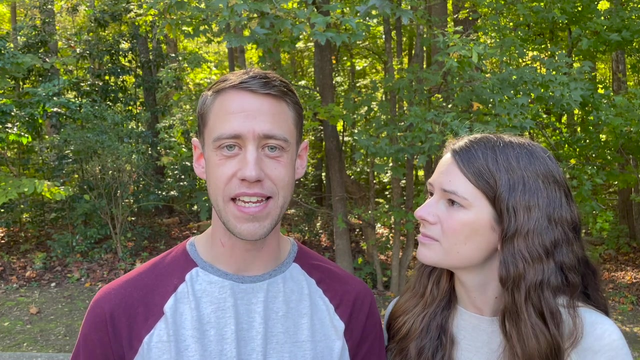 to you and not look like the surrounding homes, like you'll probably really enjoy McGregor Downs. A lot of neighborhoods like McGregor Downs will have architectural review committees And I feel like McGregor Downs does a really good job about allowing architecture that's very unique and not keeping the neighborhood like very similar. Yeah, Yeah, But in a good way. 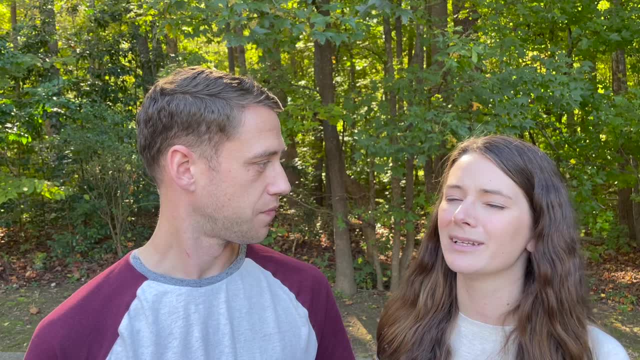 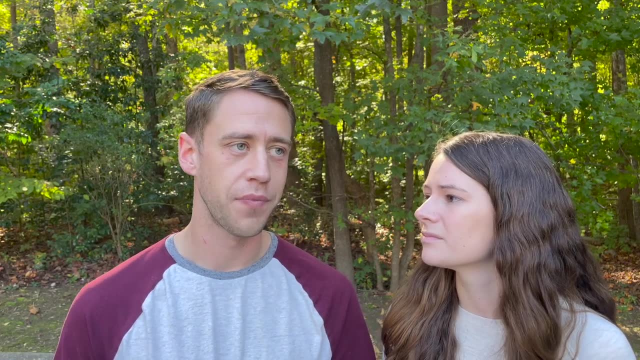 they all look like they do belong there. It doesn't? it's not like weird, It's just well done, Yeah, Yeah. And then the golf course. uh, sits on a golf course. Golf course is beautiful, Um, but yeah, I mean as far as price points go, the average in 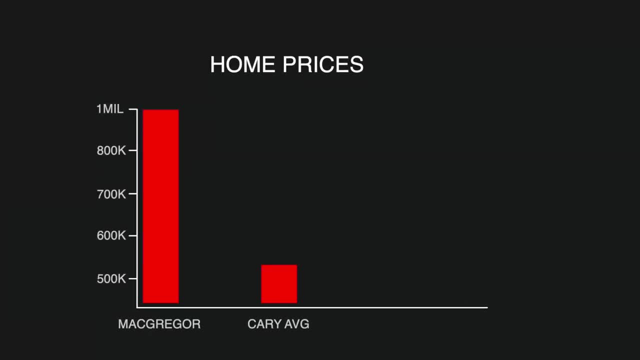 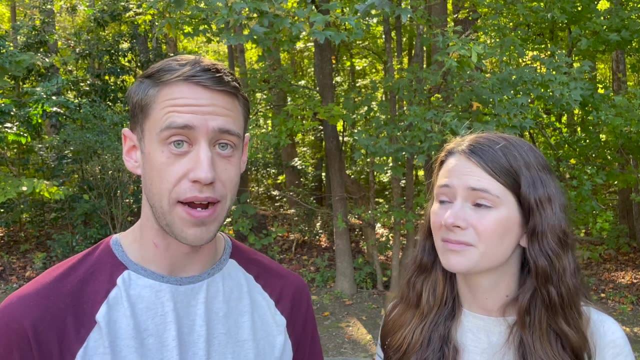 McGregor Downs is a million dollars So obviously the price point far exceeds, you know, Amberley or some of the other neighborhoods, Um, and it feels, I mean if you're driving through you can tell, I mean it's a million dollar neighborhood. Definitely When you're driving through you're 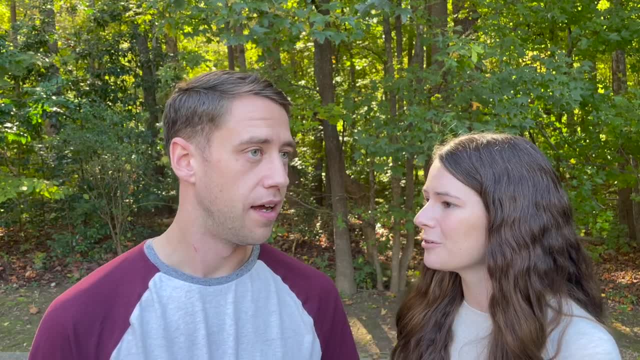 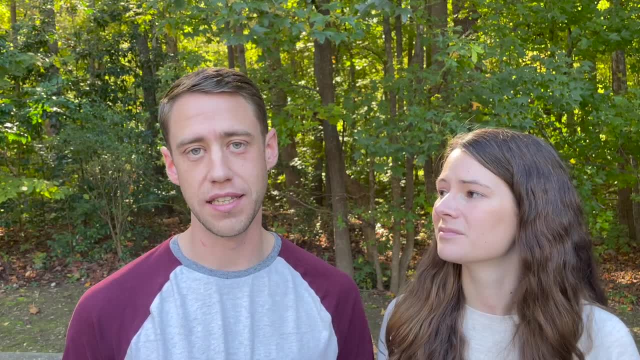 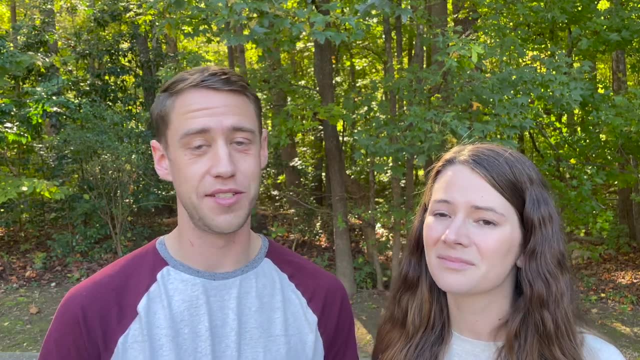 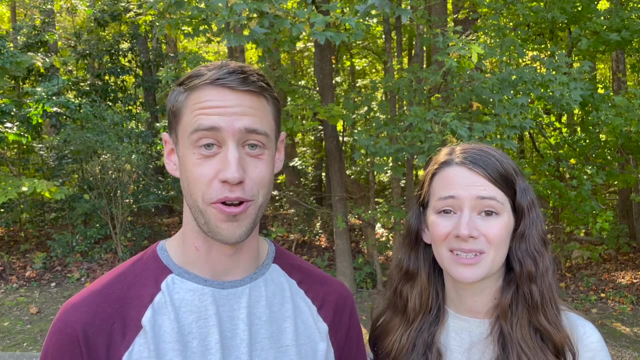 in McGregor Downs they do have townhomes, uh, those average in the seven hundreds Um. but yeah, I mean it's a beautiful neighborhood, It's near a ton of amenities, um sits on a beautiful golf course. So if, if, if it's within your budget, it's, it's great. Yeah, You can't beat it really. Yeah. So the third neighborhood on our list today is Kildare Farms. Um, Kildare Farms is going to be one of the least expensive neighborhoods we're highlighting today. It has a little bit of an older feel. It's a little bit more of a you know a little bit more of a. you know a little bit. 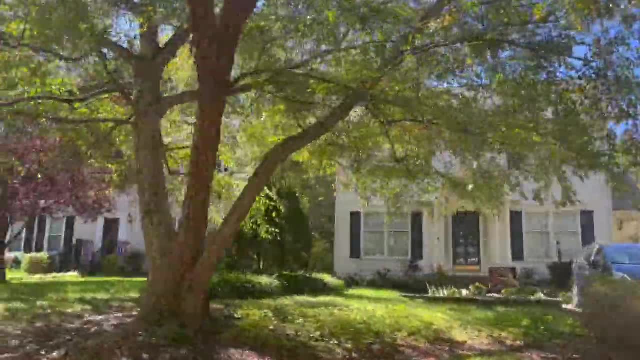 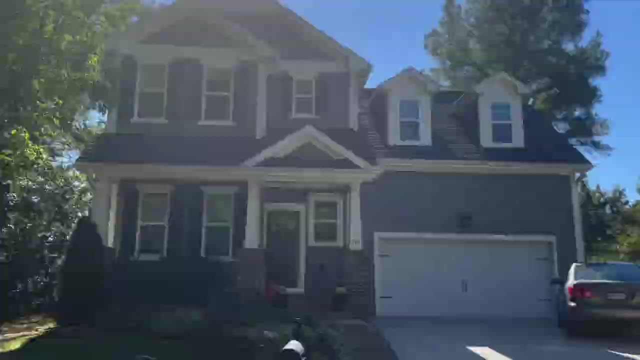 more wooded. Um. so if you really appreciate, maybe I don't know if privacy is really the right word. It's not that there's like giant lots or anything, but it just feels a little more serene and peaceful, a little less um, upkept. Definitely doesn't have the country. 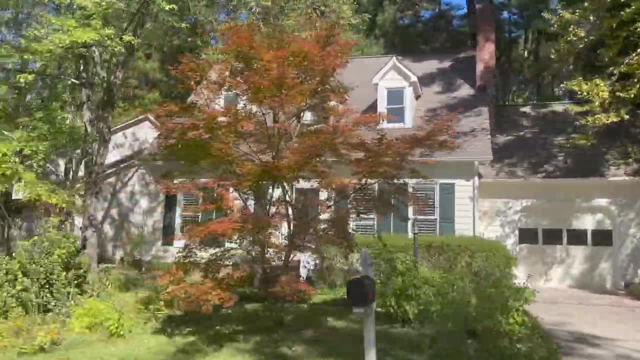 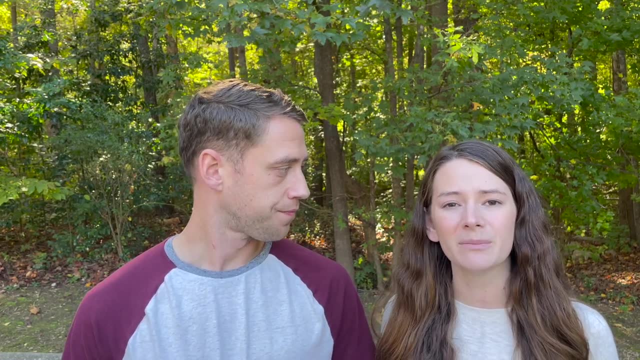 club feel that, like McGregor had, Um, but Kildare Farms it's really cute. Um, there's a lot of like attached homes in there, So condos and townhomes are pretty prevalent in Kildare Farms. Um, but there's also single family units. It has more of like a. 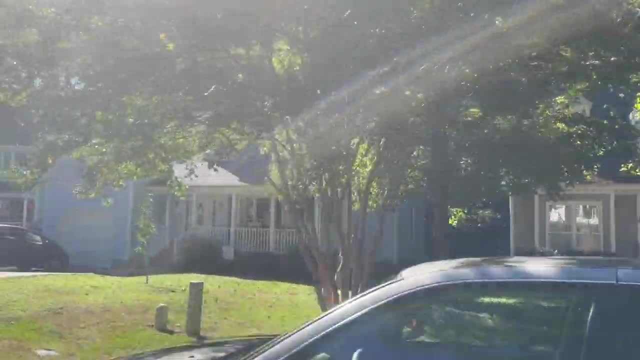 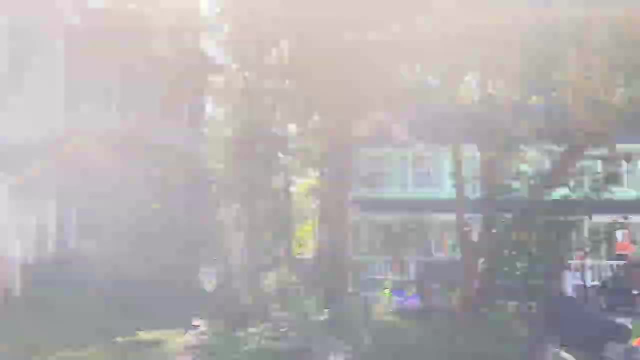 1970s type feel to it. Um for sure, maybe seventies and eighties, but it was actually one of the first planned unit developments um in North Carolina, which is pretty cool. So what that means is kind of it's just very large um sprawling. There's like shopping. 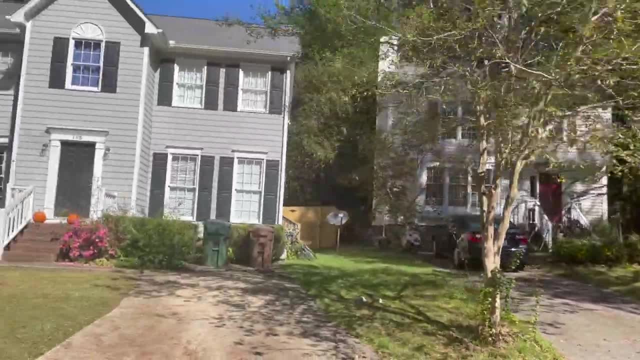 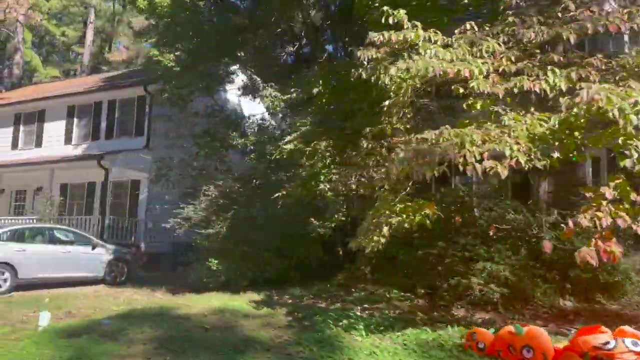 within the area. Um, just a lot to do there. There is like a, a nice pond area for recreational use. There's trails in there that are wooded, uh has a pool and everything. Not quite as fancy as the pool at Amberley, but it is still a good place to be, Um, and there's a lot of. 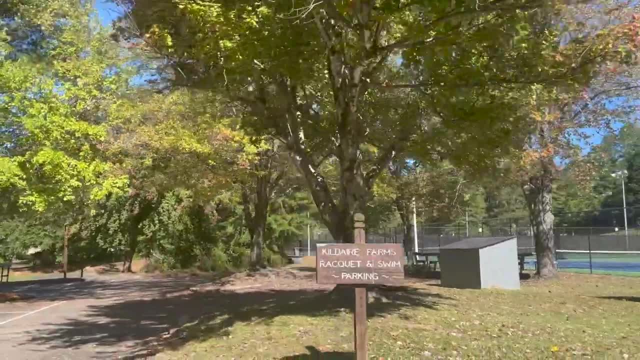 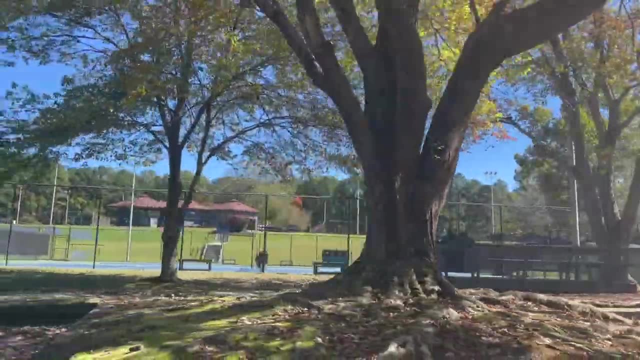 good pool for sure. Um, and yeah, like we said it's, it's close to a lot of shopping, So it's near Trader Joe's, which is pretty neat. Um, there's restaurants and stuff right across the street from the neighborhood, So that's really convenient for it. 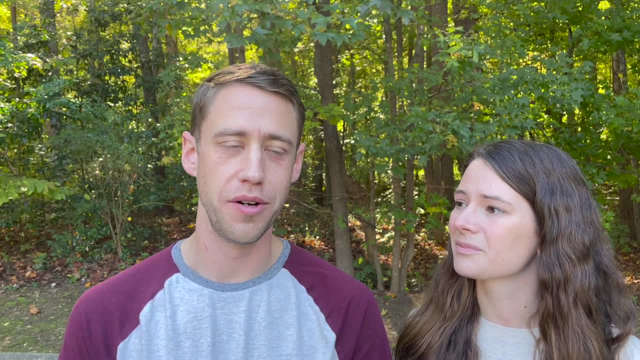 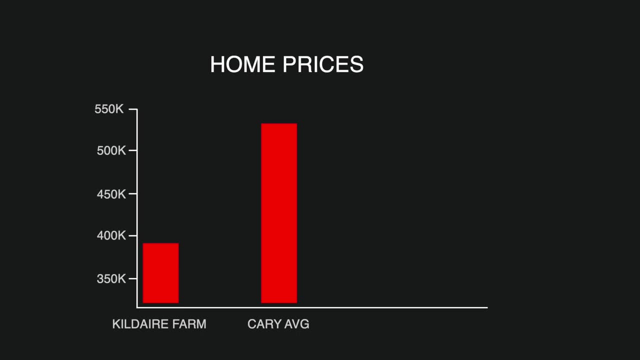 Yeah, absolutely. And as far as price points go, uh, for Kildare Farms, you're looking at average in the in the upper upper threes, um, which, for Cary is, is really really, really good. So if you want to be in Cary, uh, but the price points are a little too. much uh for, for where you're at Kildare Farm could be could be a really a really good option. So, like we mentioned earlier, average price points in Cary are about mid fives. So to come in at the upper threes is is is really good, Yeah, And it's still a. 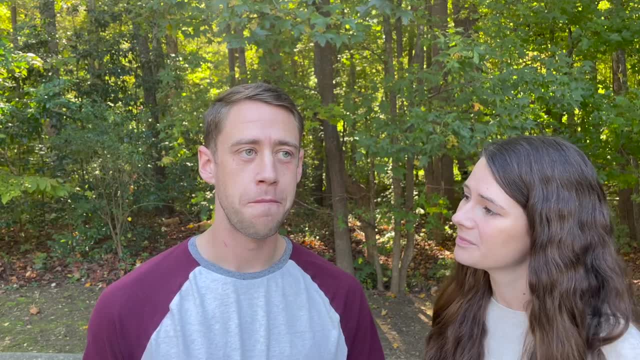 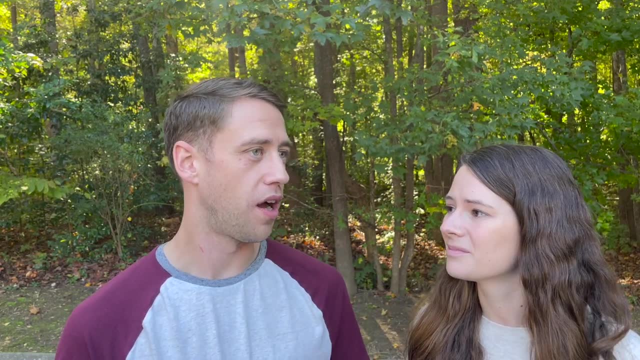 really nice neighborhood It is. It is So in in our in some of our previous videos, if you watched them, we've highlighted a neighborhood in Durham called Woodcroft. Kildare Farms is like the Woodcroft of of Cary. It's got a very similar feel to it. It's got a 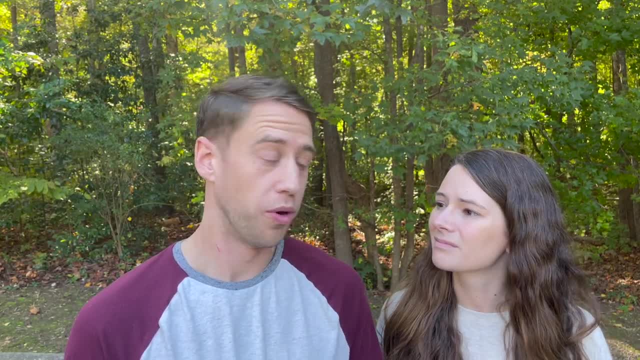 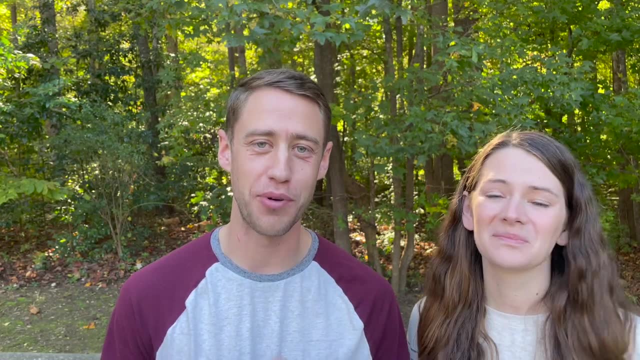 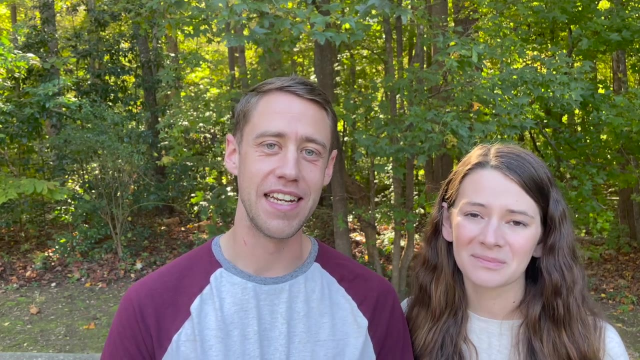 very wooded, um, but but a really a really nice, a really nice option. So all right. The fourth neighborhood on the list is Preston. So Preston's really unique in that it was founded by a company called SAS, which is located here in Cary, Um. it was founded in. 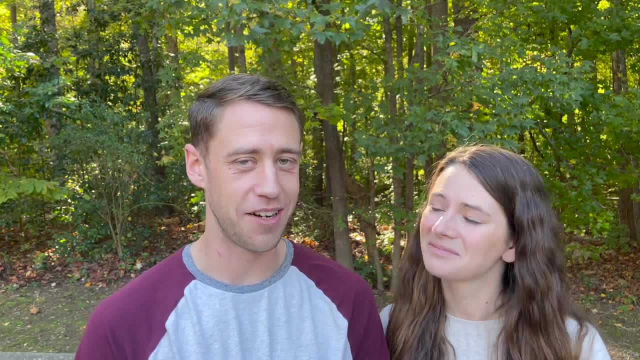 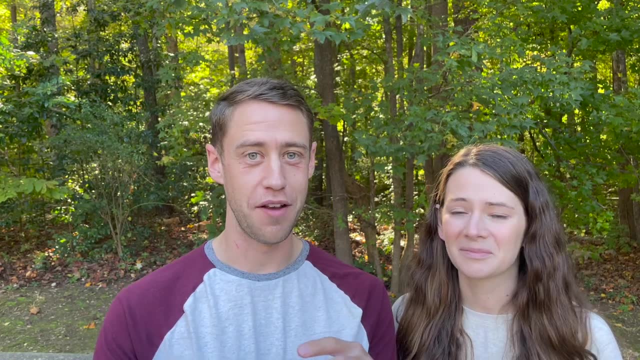 the early nineties. I just think it's really cool. Growing up I grew up near a town called Baden and there was an aluminum factory called Alcoa and they basically founded Baden. So I don't know. It's kind of cool that a company would do that, But anyway, 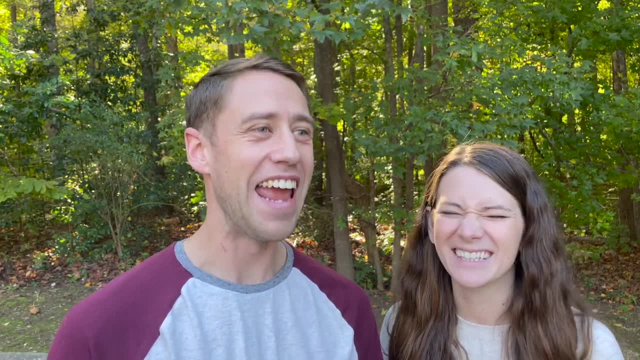 that's besides the point. Preston's a little nicer than than Baden It is, but it's a similar. it's a similar concept. I don't know It's really it's, it's, it's really cool, But uh, yeah, But. 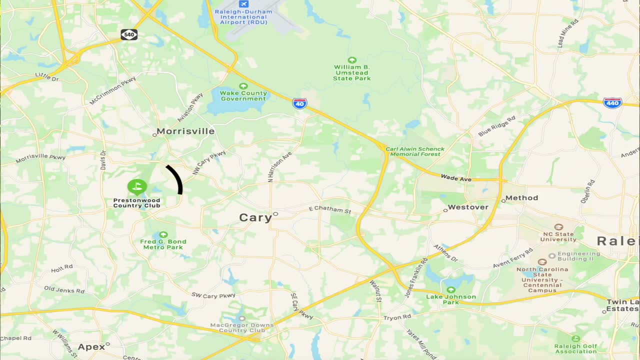 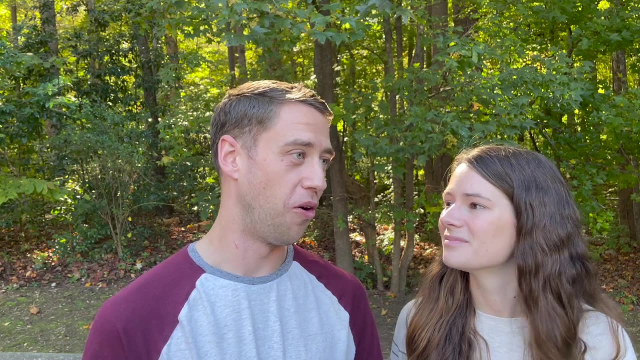 anyway. so it's on the West side of Cary, Um, and just it's on, it's a country club Um, tons of beautiful homes, I mean it's just, it's a, it's a stunning neighborhood. Yeah, If I had. 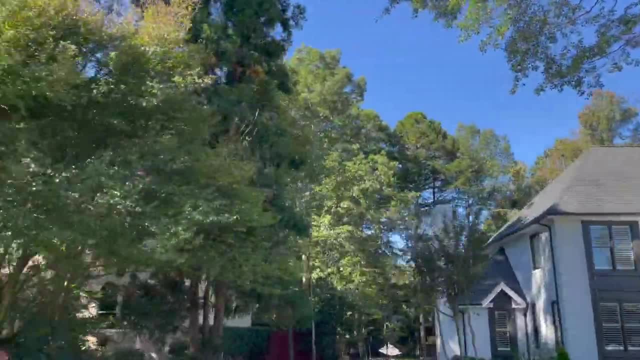 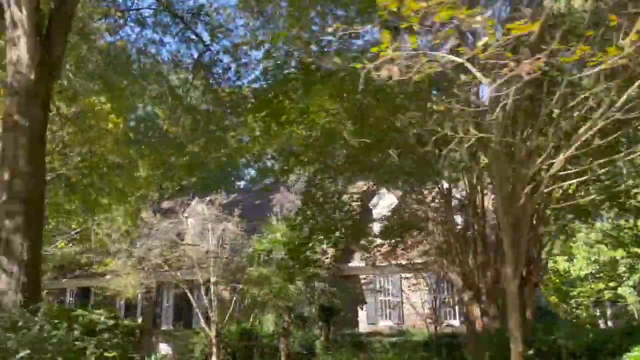 been looking at. I would say it's probably the closest to the McGregor Downs um neighborhood, but I think in general the- I mean it's very manicured in the same way that McGregor Downs is, but I think maybe the home sizes are a little bit smaller. Um, not all of them, but the price. 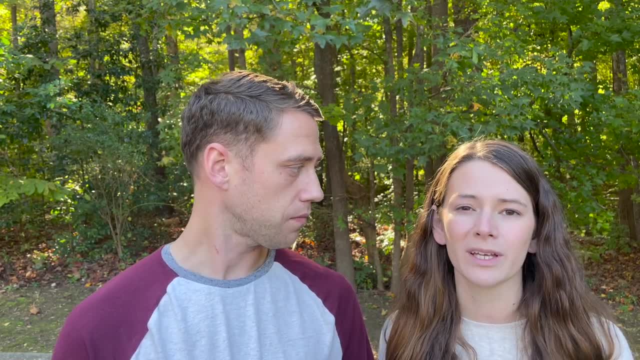 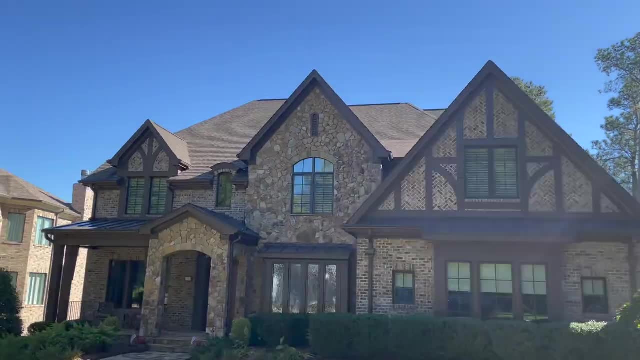 points come in a little cheaper, Um, so a little bit more affordable than McGregor is, but you still get the same kind of feel as McGregor, where you have more stately homes and also have the golf course and the country club type feel. Yeah, So price points in Preston are going to be um in the 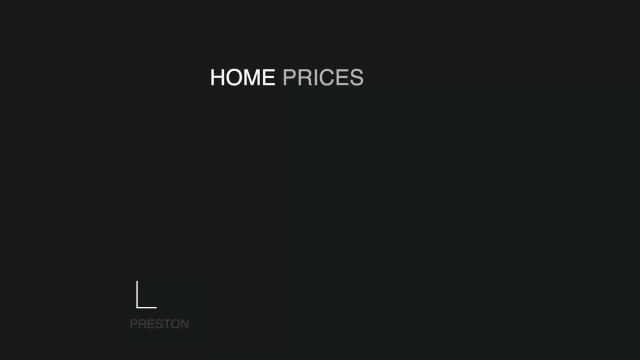 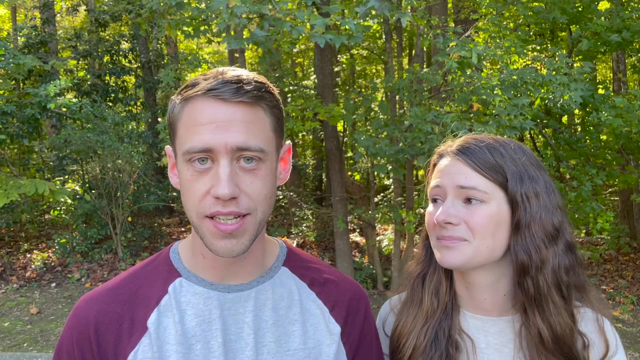 average in, in in the seven hundreds Um, so obviously that's above average in Cary, Um, but it's. I mean, it's a gorgeous. it's a gorgeous neighborhood. It's near a ton of amenities, just like pretty much every other neighborhood in Cary is Um. so there is a uh, there's a. 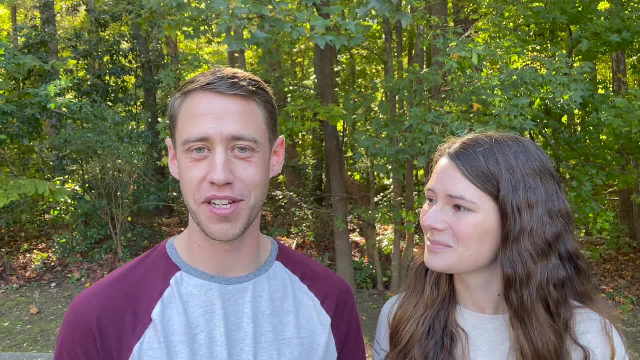 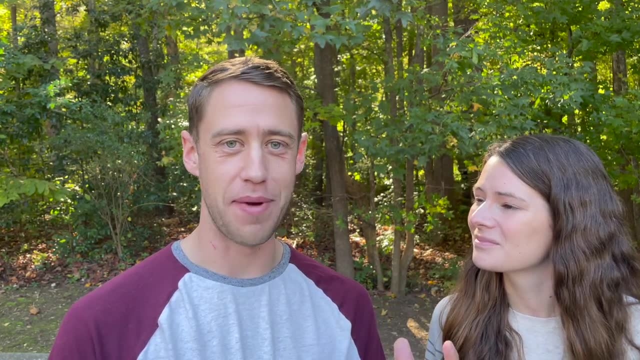 crumble cookie nearby and I don't know if you've ever had crumble cookie. Didn't it originate out West? Yeah, I think in Utah or something, Yeah, So basically there's these cookies and they're like the size of my head and they're, they're just, they're incredible. 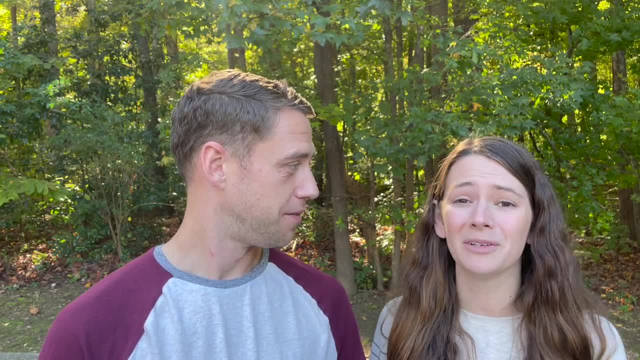 So good, They're incredible. They're so good. Yeah, It's hard to describe it really, but if you have one nearby you, you've got to, you've got to try it, Yeah. So I don't know, I'm just pointing. 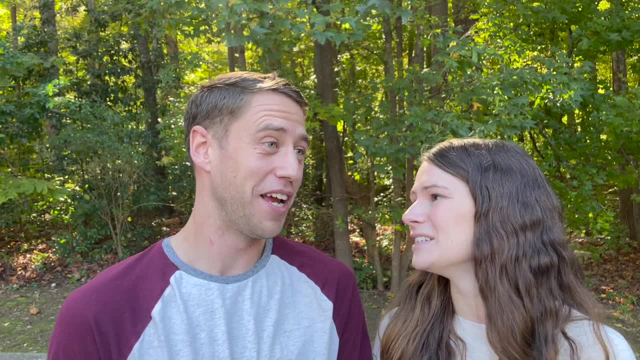 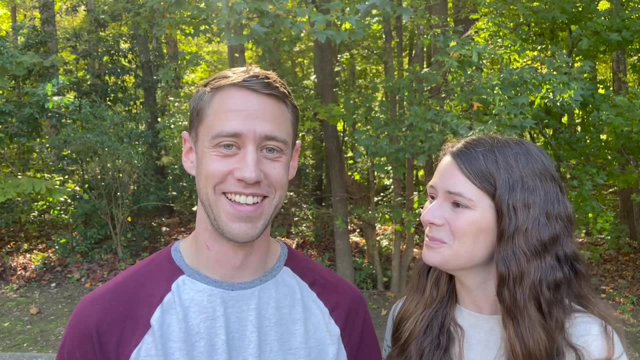 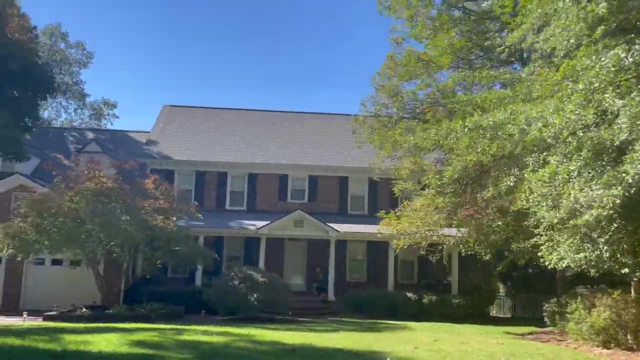 out one random restaurant in that area, but it's, it's really. it's a really good. it's not a reason to move to Preston, obviously, but it's really. if you like cookies, might as well. So the fifth one on our list and the last one for today is Lockmere. Um Lockmere. I always come back to it as probably. 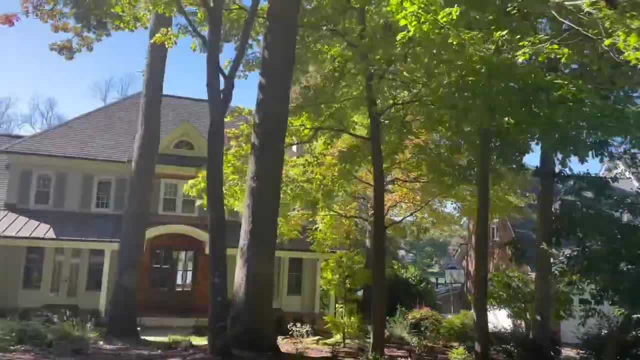 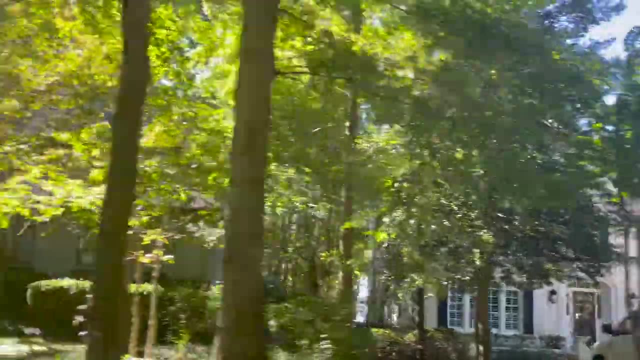 being one of my favorite neighborhoods in the whole triangle. It's just it has a unique feel to it. Um, it's kind of like a mixture of Kildare farms and McGregor towns, I don't know- like it's wooded feeling and very like you can enjoy nature, cause there's a beautiful like lake there- Yeah, The. 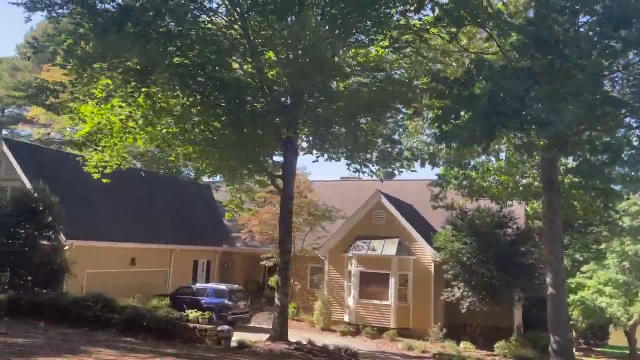 lake's amazing. It's so pretty And so there's just a lot of trees, Um, but the homes are kind of nicer. I don't know how to explain it, but it's just gorgeous. I love the feel of it. It has a lot. 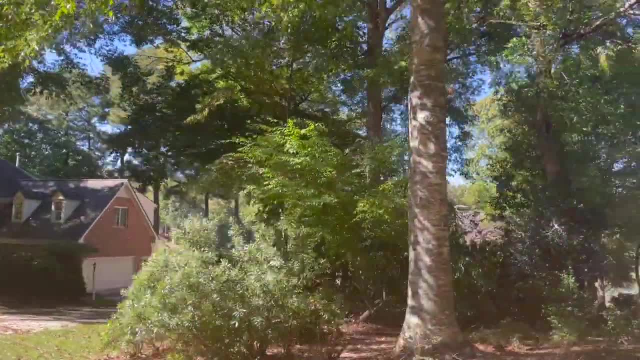 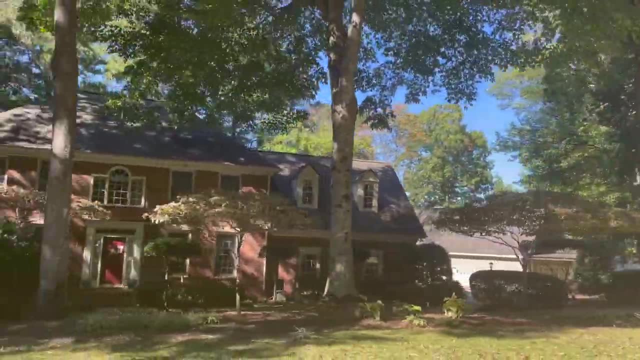 of character and charm that I think is missing in not I think all these neighborhoods have a lot of character and charm, but you don't see it in every neighborhood everywhere, And so anytime you go to Lockmere it just feels special. Yeah, Yeah, Lockmere's, Lockmere's selling point, I feel. 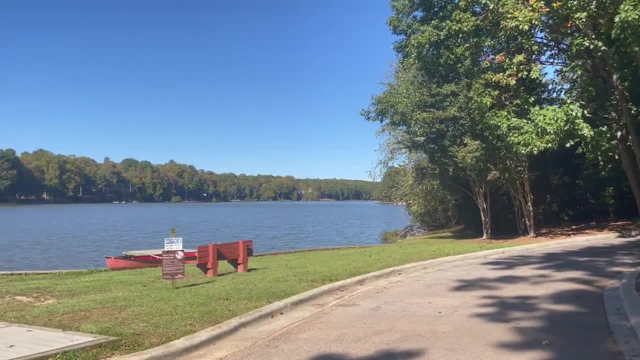 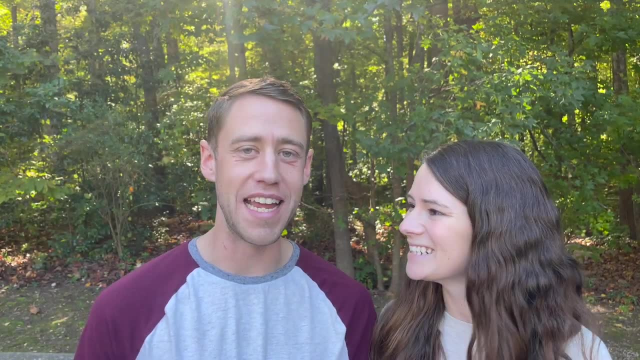 like is is the lake. Yeah, And the fact that you can have a house on on a lake, I I mean, I wouldn't call it a lake, It's more like it's more like a big pond, but but but they call it. 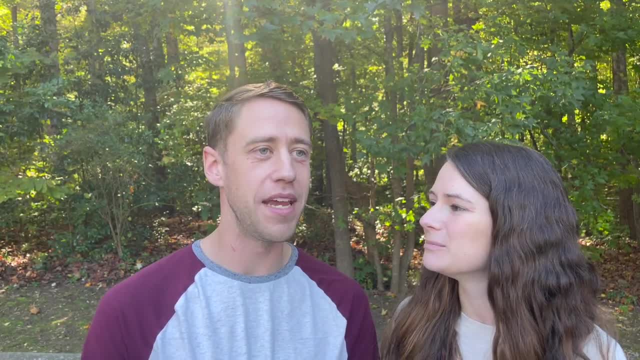 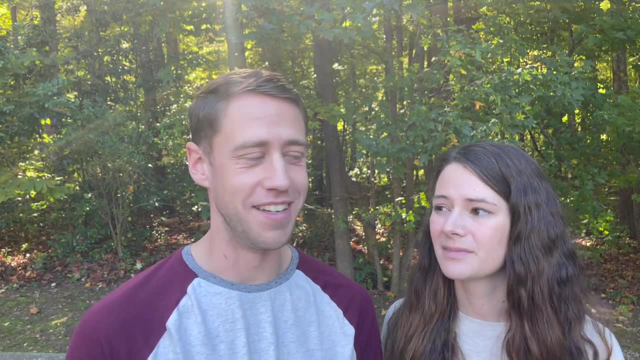 a lake. So I'll, I'll, I'll, I'll use their language, but I mean you, I mean you could put a boat in it, Um, and so you know, it's a, I mean, it's a good size. it's a good size pond. 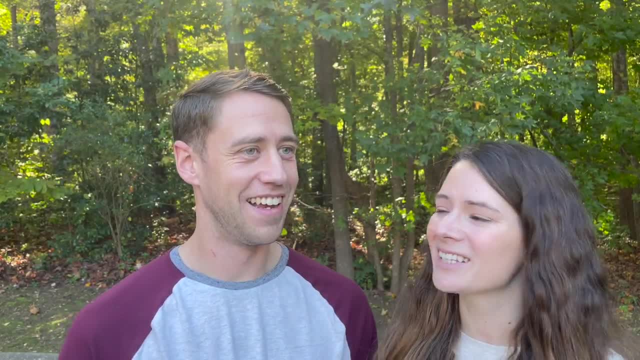 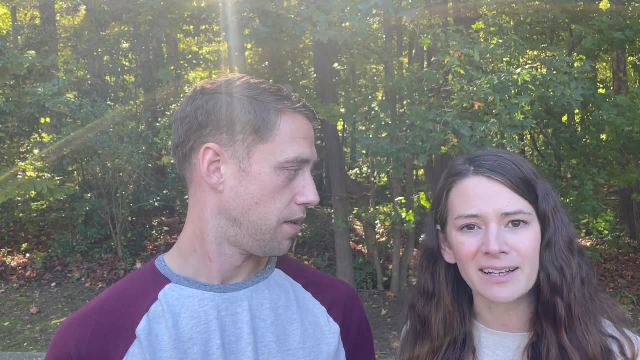 Yeah, You know good size pond, Yeah, Um yeah. And, like Zach said, there are homes that do face the lake. So there are options to like actually have the lake be in your backyard, and tons of homes don't have that access, but they still can access the lake. 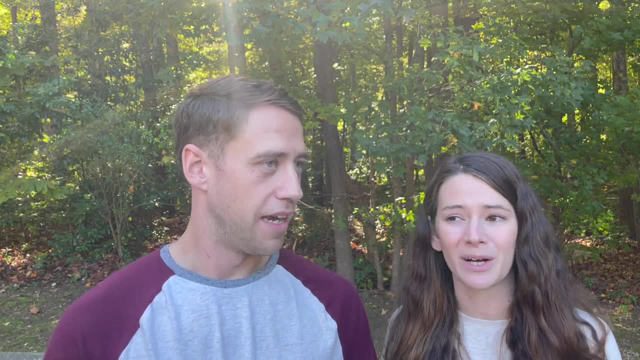 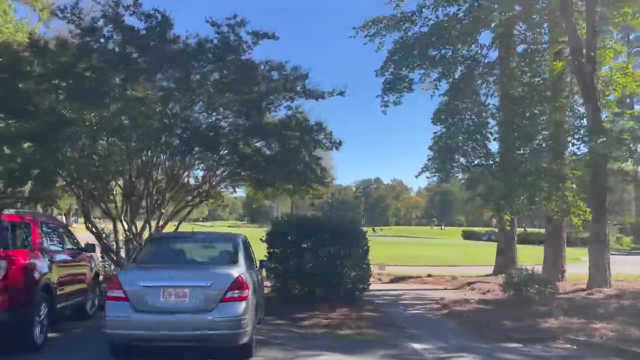 There's like docks and things like that to get to it, and walking trails around the lake, So just really nice and peaceful. Yeah, it is, And there's a golf course that is off to the side, uh, in Lockmere. Um, it's really nice country club as well. Uh, there's a couple of playgrounds. 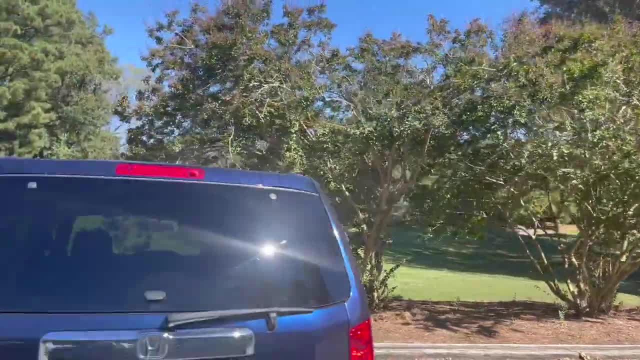 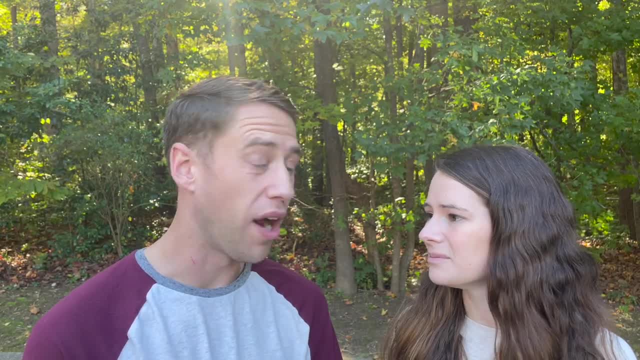 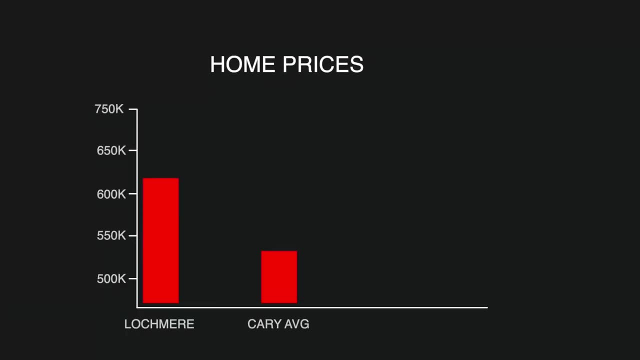 very well manicured. Yeah, It's, it's, it's beautiful. So price points in Lockmere are going to come in, uh, on average in the low sixes, Um. so you know, that kind of puts it slightly above. 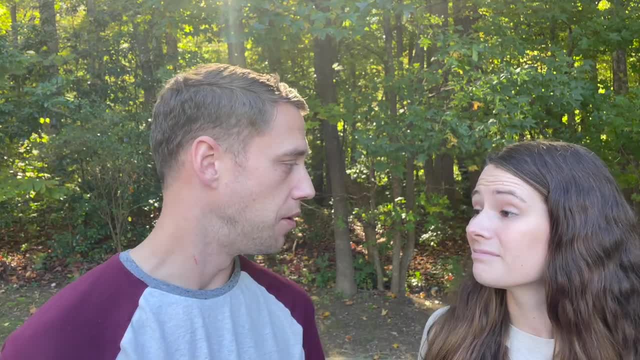 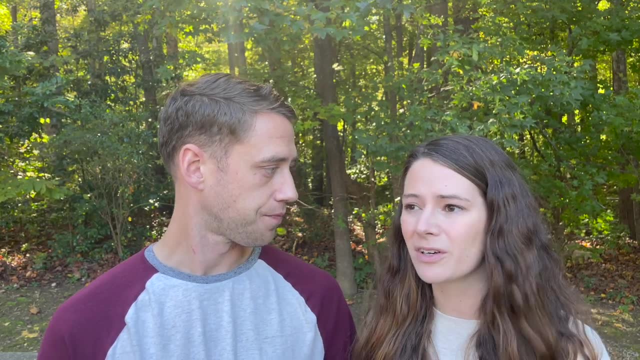 average, uh, in Cary, but but pretty, pretty close, pretty close to the average, the average mark Definitely. And there are a lot of different types of housing. in Lockmere, You know you have homes that just feel kind of basic isn't the right word- but just traditional, normal looking homes.